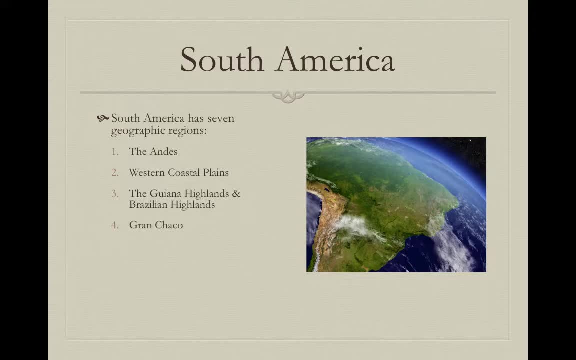 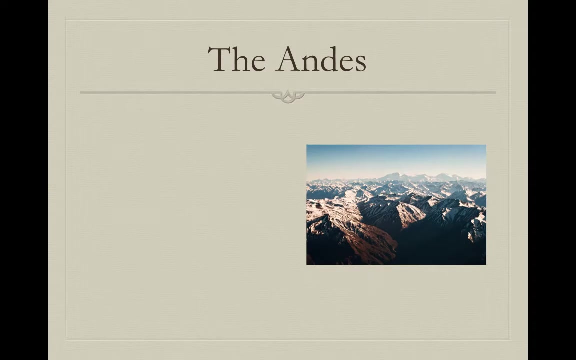 Brazilian Highlands, the Gran Chaco, the Pampas, Patagonia and the Amazon River Basin. At 4,500 miles in length, the Andes is the longest mountain chain in the world. Aconcagua is the highest mountain outside of Asia, at 22,834 feet. 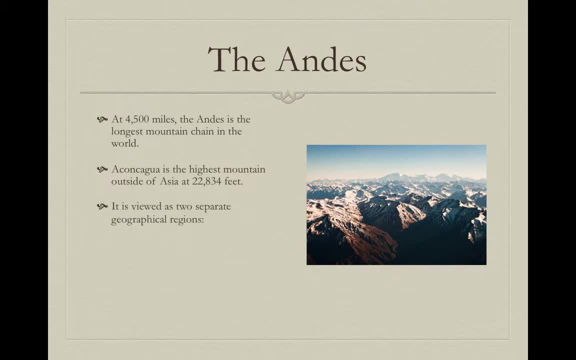 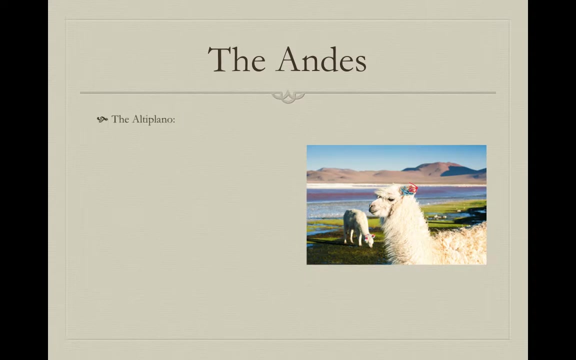 It is viewed as two separate geographical regions: the Altiplano in the northern Andes and the Sub Mountain, the Umpire. For one, it is the highest mountain chain in the world. the sub mountain region in the south, The Altiplano, consists of several highland. 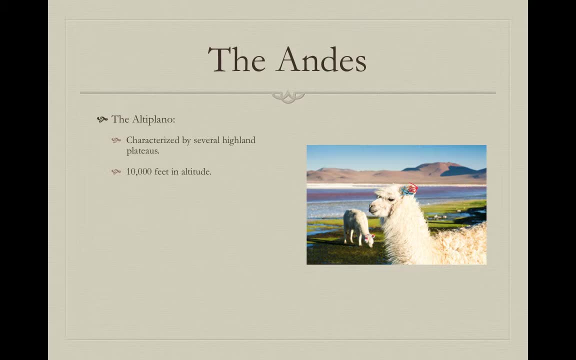 plateaus, and it is at an altitude of about 10,000 feet. It has rich soils that produce crops. The sub mountain region has lower elevations, forests and slopes, and extends to the southern tip of Chile, The Western Coastal Plains, Located between the 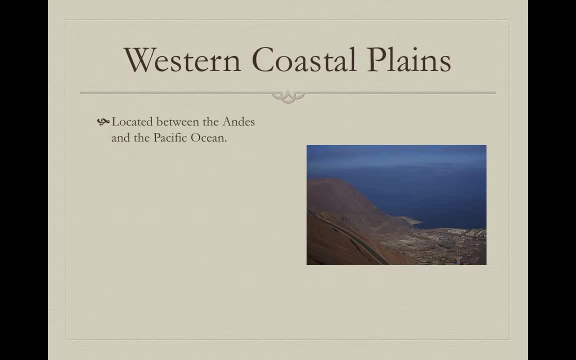 Andes and the Pacific Ocean are the Western Coastal Plains. They extend from Panama southward to Peru. They are lush green land and have a humid climate. South of Peru, it gives way to the Atacama Desert, which is the driest desert on earth. The Amazon River Basin. The Amazon River. 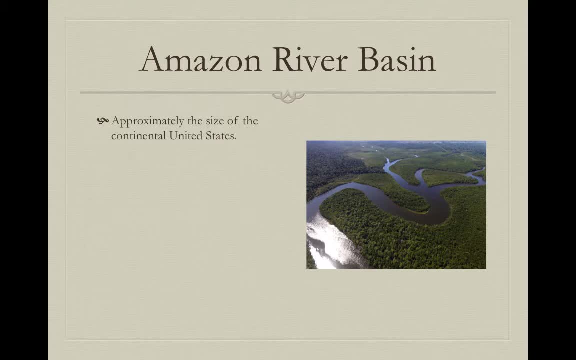